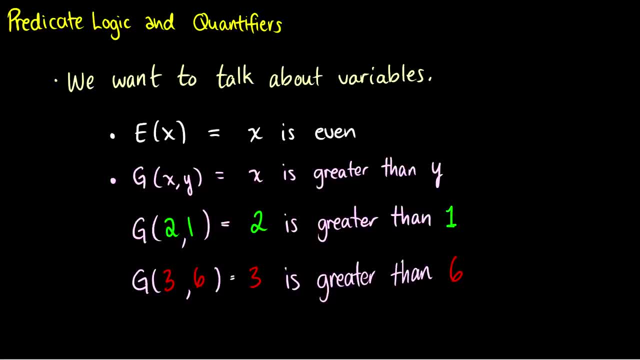 In this video we'll talk about predicate logic, quantifiers and negation. So what is predicate logic for? Well, we want to talk about variables. So before we couldn't have a statement like x is even and then just plug something in for x. That wasn't possible in. 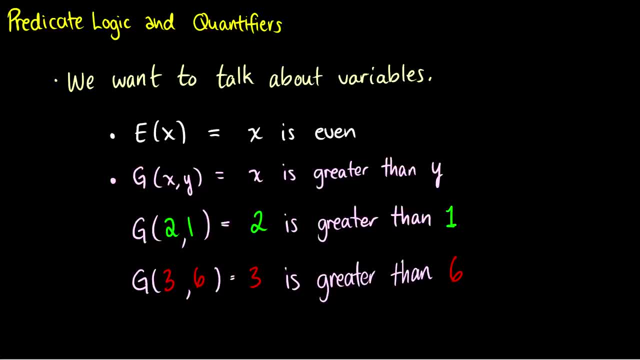 propositional logic. But in predicate logic it's now possible because our predicates also have terms. So a predicate looks like ex, and this is the proposition, or predicate x is even. Another example would be a two-place predicate, gxy, which could mean something like x is greater. 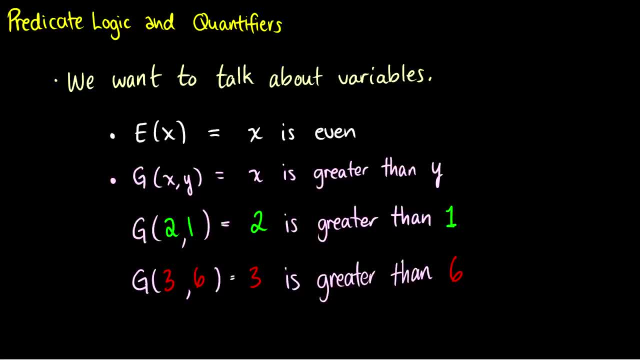 than y, And these are variables, But we can stick in these constants as well. So g21, if we just ignore this, x is even thing here. if we have gxy, x is greater than y. if we plug in x, we get a predicate that looks like ex. So we can stick in these constants as. 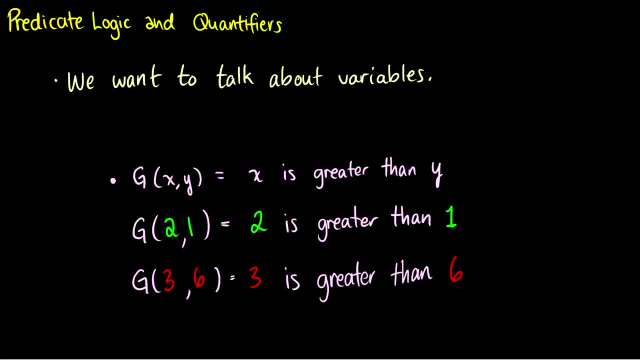 well, So g21, if we just ignore this, x is even thing here, if we have gxy, x is greater than y, 2 and 1 in that says that 2 is greater than 1 and this has a truth value. so 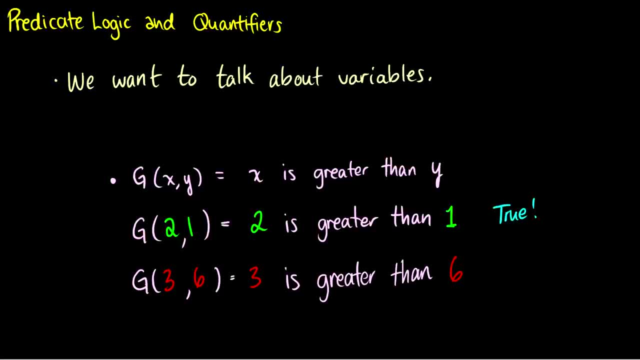 this statement is true, but if we put 3 and 6 in there- for 3 is greater than 6- then this predicate is false. now, what's different between these closed formulas and this open formula? well, closed formulas have truth values and open formulas do not have truth values. therefore, this G is not a statement. 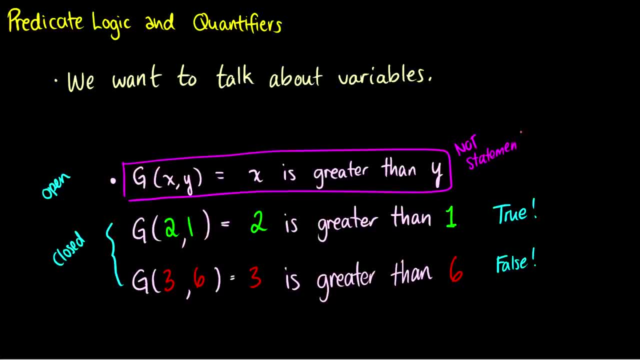 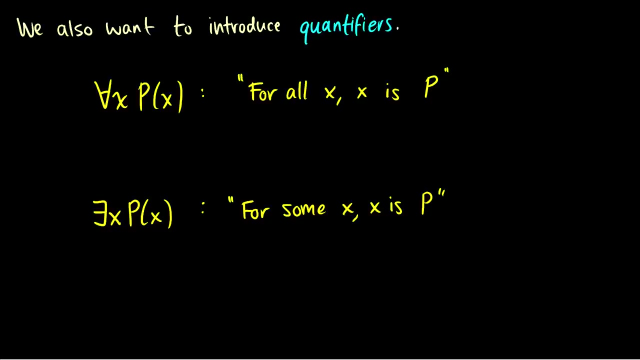 which means we can't even have it in propositional logic at all. we need predicate logic in order to say something like G is greater than Y and assign truth values to constants plugged into those variables. and that's one thing predicate logic lets us do. but the more important thing it does is it gives us quantifiers. and this is the 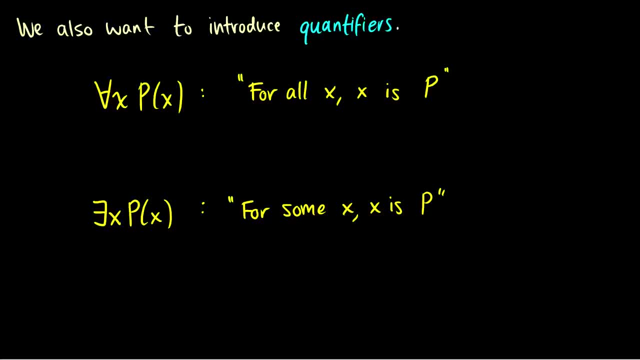 upside-down a and the backwards e. so the upside-down a is known as the universal quantifier, and for all X, P X. it's kind of read as for all X, so this is for all X and then P X, so it's gonna be for all x. X is P for all x, x is happy something. 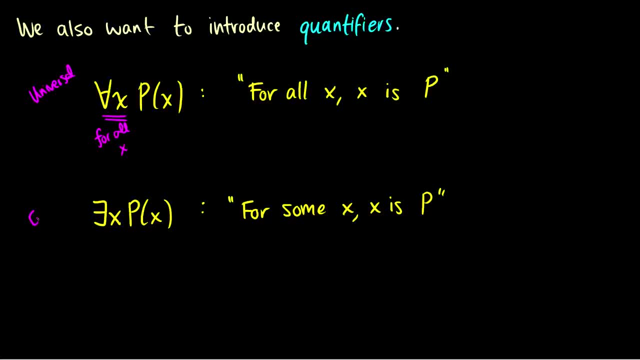 like that. now the backwards e is known as the existential quantifier and this says there exists at least one x, so we could say there exists x. or another way to say: it is for some x, so exist. XPX could be read: as for some x, x is p. Or there exists an x such that x is p, So there is some x, such that x is happy. 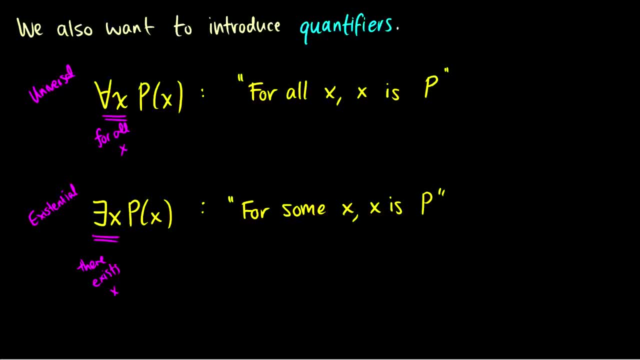 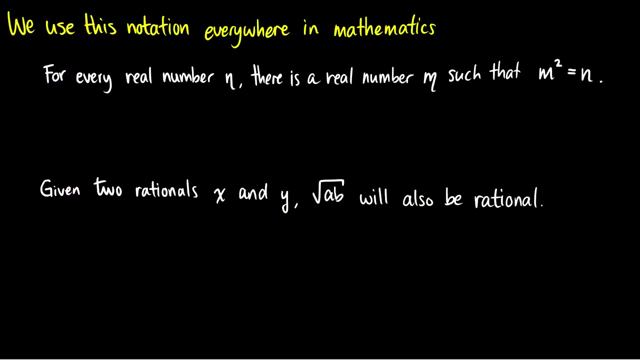 And quantifiers really give us much more strength when translating sentences into English, as well as looking at truth conditions for certain English sentences, certain scenarios or even mathematical operations. So we use this notation everywhere in mathematics. So I'm going to convert some English sentences, well, some mathematical statements, into predicate logic. We're going to 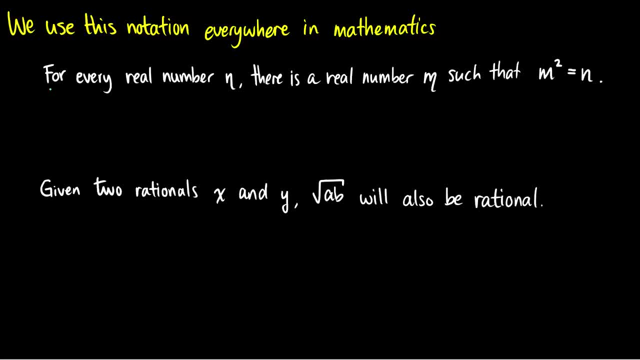 take it step by step. So the first step, I'll read it out: For every real number n, there is a real number m such that m squared is equal to n. Let's not focus on the proof or whether it's true. 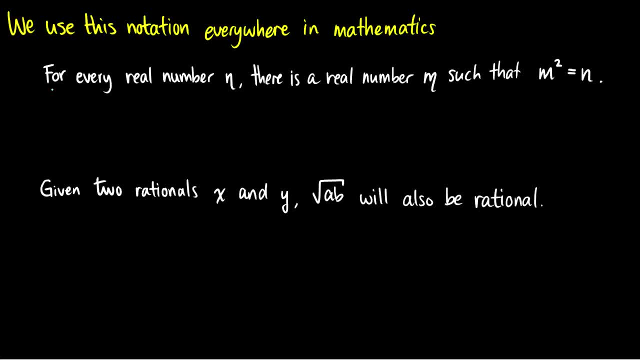 let's just translate this into predicate logic. So for every real number, n for every number. this is the universal. So we're going to have for all n, and these are real numbers. so for all n in the set of real numbers. 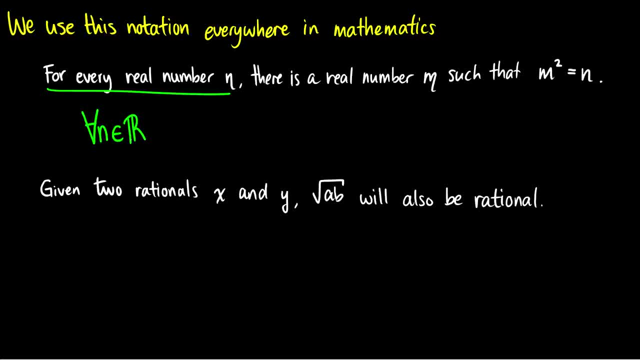 so again, for all n in real numbers- you should remember this from set theory- there is a real number m, So there is a real number m, there's at least one, So that's the existential. so there exists an m in the reals, such that and then m squared is equal. 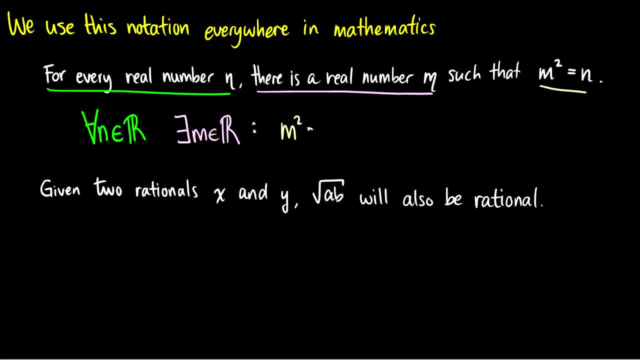 to n. We can just leave this the same thing, so we can say m squared is equal to n, or we could say pmn, and then we could define that being m squared is equal to n. Either way works Typically. we would just write m squared equals n afterwards. So for all real numbers, n, there is a real number. 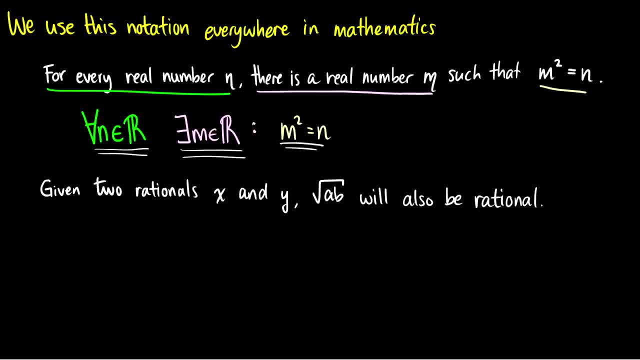 m, such that m squared is equal to n. Let's take a look at the second one. Given two rationals, x and y, the square root of xy will also be rational. Now, this doesn't look like there's any univariate rationalization here, but it does look like there's any univariate rationalization here. 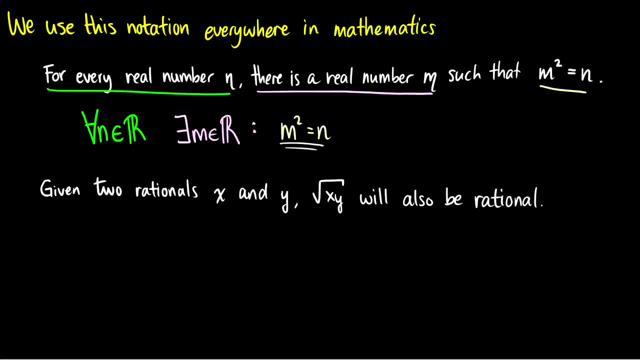 But there really is one here in disguise. So, given two rationals, x and y, what this says is: given any two rational numbers. So this is for all x, y in the set of rational numbers, which is the q, there The square root of xy will also be rational. So we can just say: and the square root of xy is also. 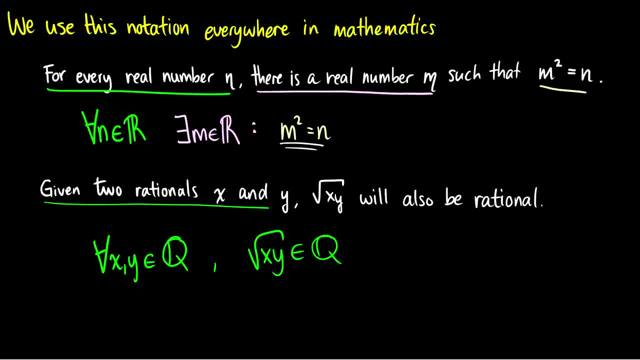 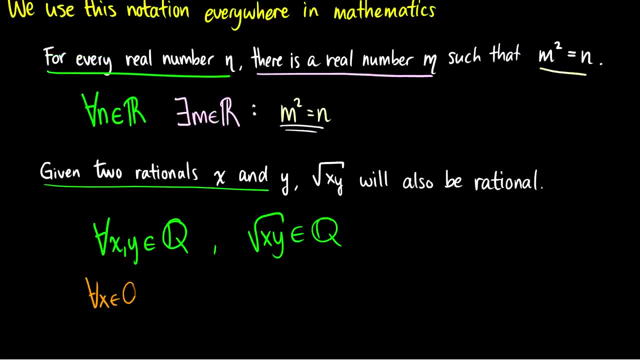 in q. So this is another way of abbreviating things. So I wrote for all x- y in q, but you could also write for all x in q, for all y in q. either way, They're both exactly the same thing. One is shorter than the other, but there's no difference. 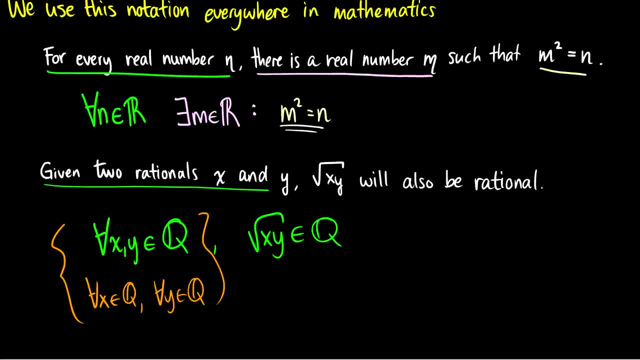 when they have the same quantifier. So that's translating some mathematical statements into predicate logic, And it's important to be able to go both ways, to be able to translate it into predicate logic and to be able to read it and understand it. But let's talk about negating quantifiers. 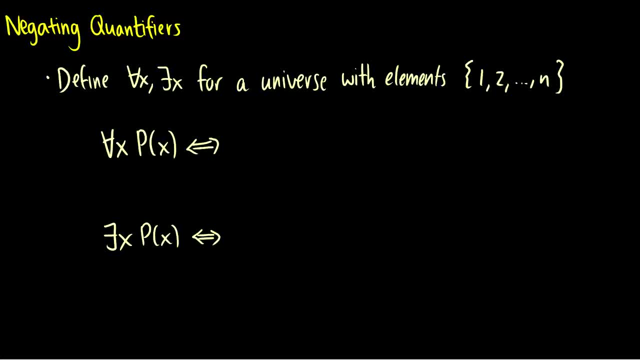 since this is usually the tricky part And I really want to define for all x p x and their existence in x p x in terms of propositional logic in a way, So we can kind of see how negation really looks like under the surface, So in the deep structure. 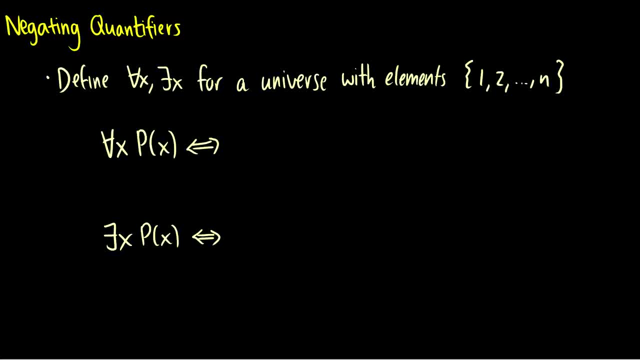 what's happening. So I'm going to have a universe with elements 1,, 2, all the way up to n. So for all x, p, x. when is this true? This is true if every x in the universe is. 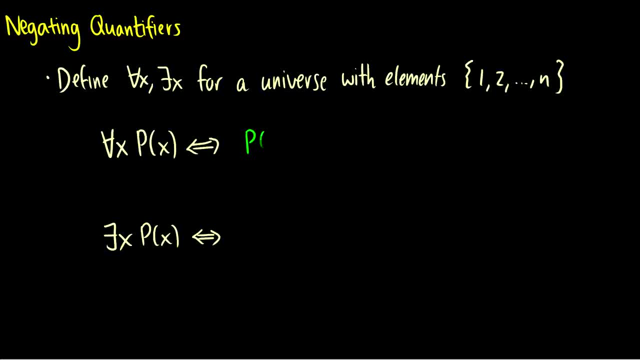 p. So this is like saying p 1, and p 2, and all the way up to p n. So if all of those are true, then all x p x is true. What about their existence in x p x? Well, that's. 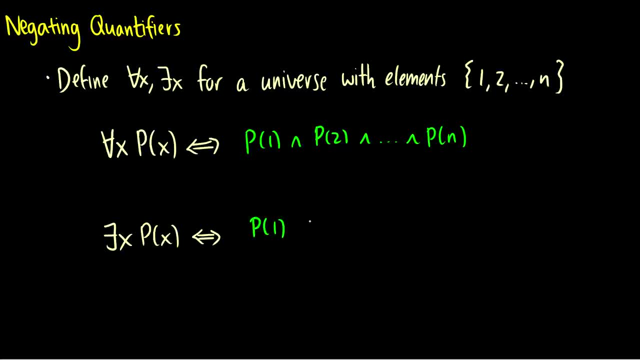 saying at least x, p, x is true. So if all of those are true, then all x, p, x is true. So this is like saying p 1, or p 2, or all the way up to p n. So that's really what. 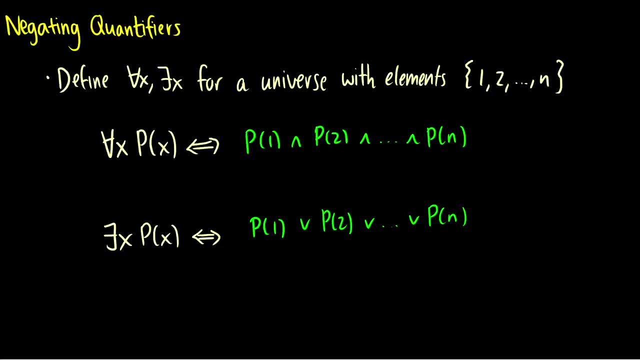 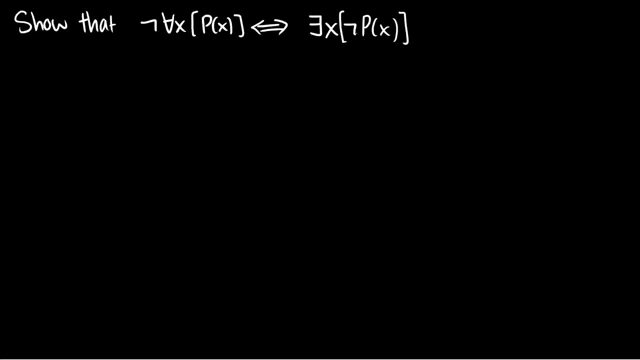 all x, p x and exists. x, p x means. Now, when we negate these, we'll be able to see how negation works using these definitions. So let's show that not for all x, p x is logically equivalent to exists. 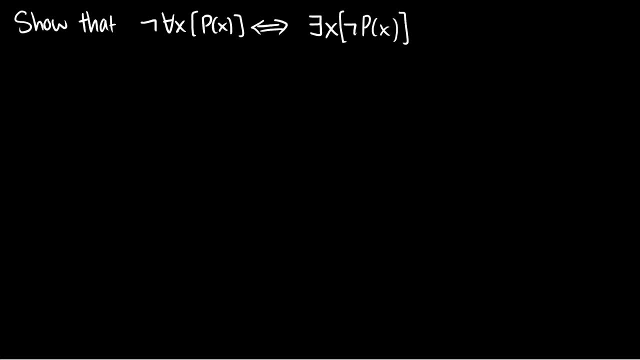 So first I want to start out with all x, p, x, and I want to write the definition again. So this is like saying p 1, and p 2, and all the way up to p n. Now, if we negate this, 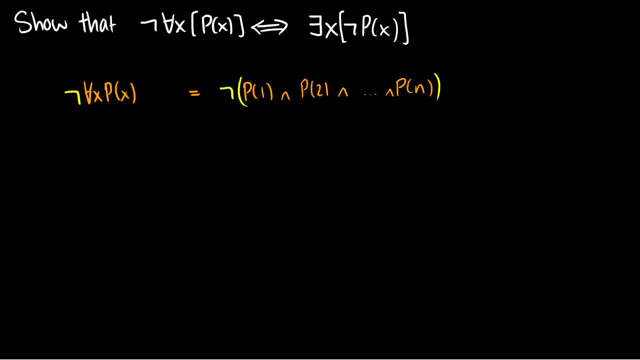 then we're really negating this whole thing here, And with the Morgan's Law we can distribute that negation. So this is like not p 1, or not p 2, or dot, dot, dot all the way up. 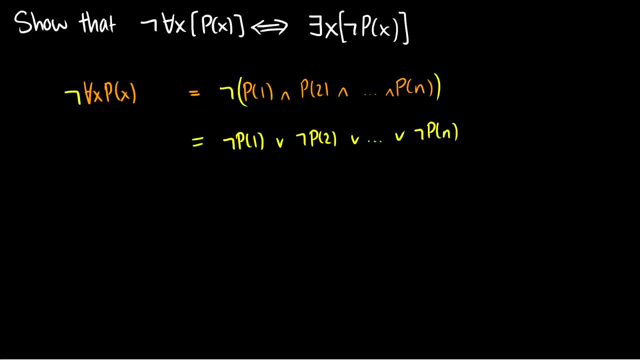 to not p n. Now, what does this look like? Well, this kind of looks like there exists an x, except, instead of just having p x, we have not p x Because, remember, if we're looking at the definition of exists in x, so exists in x, p x, is just p 1, or p 2,. 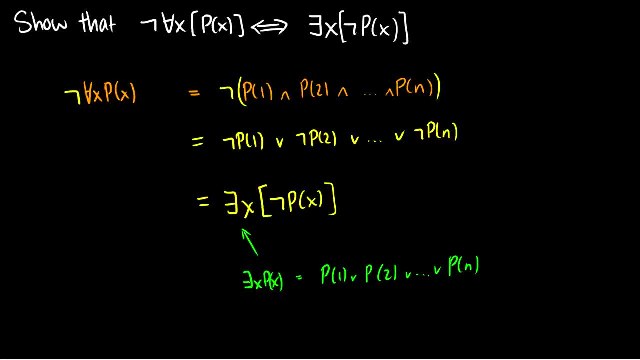 or all the way up to p n. Now these look very similar, except there's just a negation in front of each term, which is why we have the negation in here. So not for all x. p x is the same thing as there exists an x, not p x. 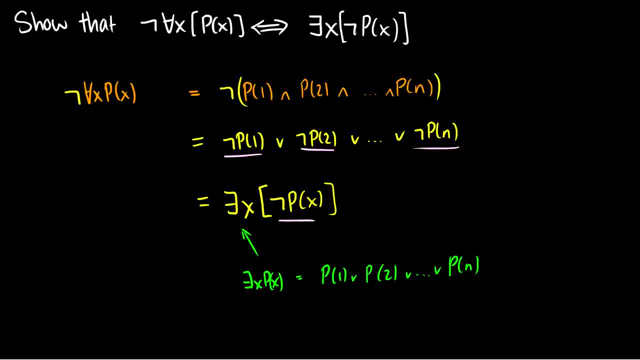 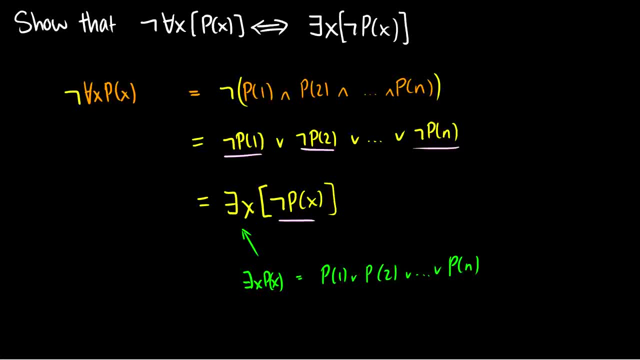 Not all dogs are brown. That means there is some dog that is not brown. So all dogs are not brown means that there is some dog that isn't brown. So that's a nice English way we can talk about the logical equivalence between the negation. 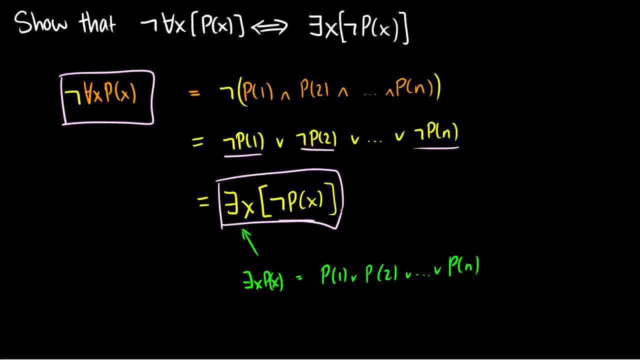 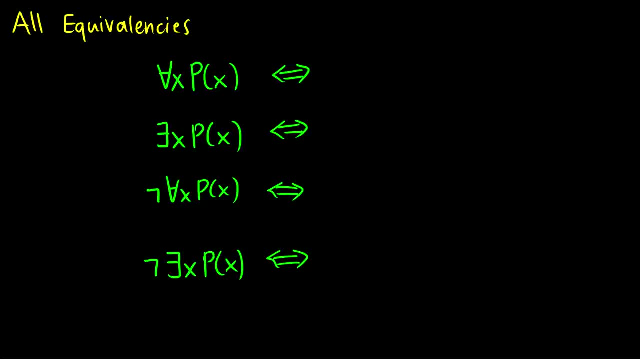 of these universals and existentials. In fact, there's four equivalencies. I just did one and I encourage you do the rest on your own, But we can see that all x px is the same thing as not existent x, not px. 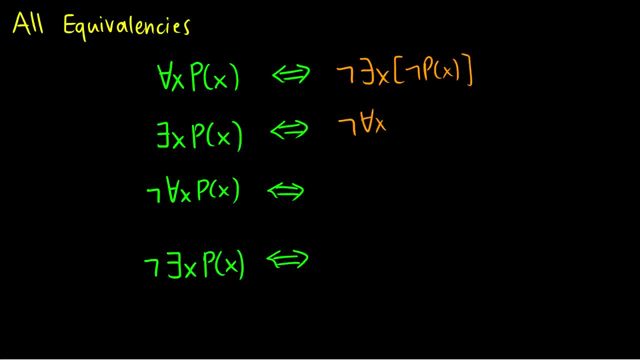 Existent x px would be the same thing as not for all x, not px. And again, using the definitions, we can show these. So I encourage you, on your own, to try with the definitions showing that these are true. Not all x px, we just did this one. 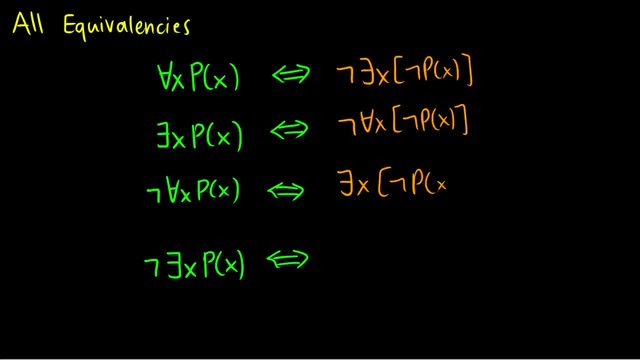 This is the same thing as existent x, Not px. And finally, not existent x px would be the same thing as for all x, not px. And you might be wondering: do I have a sheet on me that tells me these equivalencies? 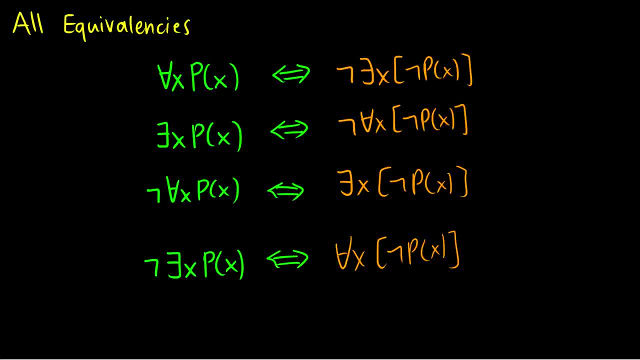 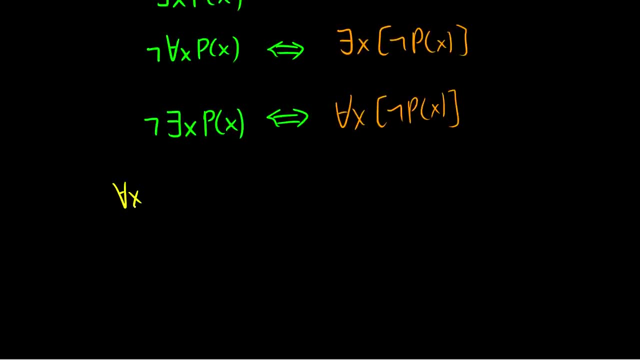 Did I memorize these Or is there some trick for this? Well, there is kind of a trick here And let's think of for all x. Actually, let's think of the one that we did For not all x, Px. 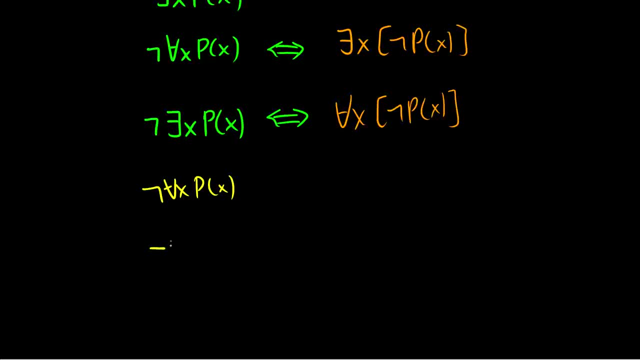 I'm going to rewrite this as not all plus p. So of course, the px I've reduced to p, The all x I've reduced to all. The negation I've written as a minus, And the fact that there's no negation there I wrote as a plus. 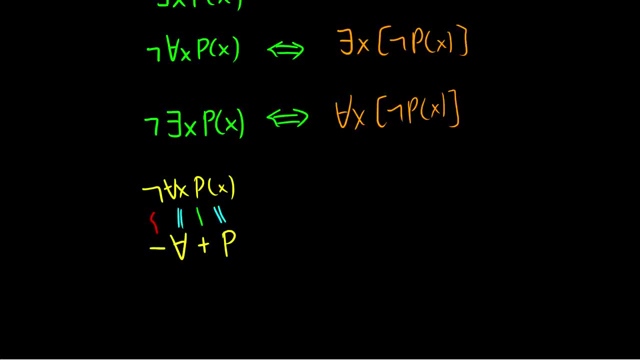 So how do we get the logical equivalence? Well, we just reverse the negations And pluses And change the quantifiers. So if we were to write this: not all plus p, as plus exist minus p, Then we can translate this back to existent x. 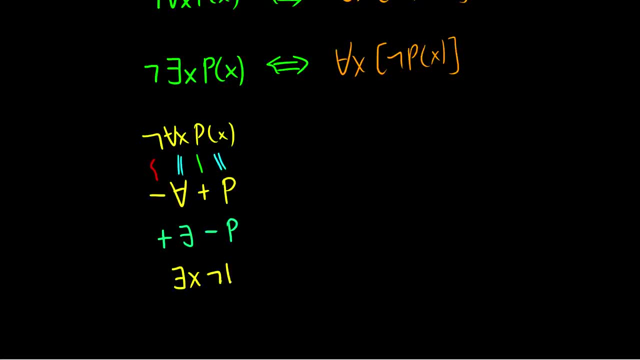 Because the plus just means no negation, Not px, And these are logically equivalent. Let's do the other one. So let's find a logical equivalent to Existent x px. Okay, first let's rewrite that So that is: plus exists plus p. 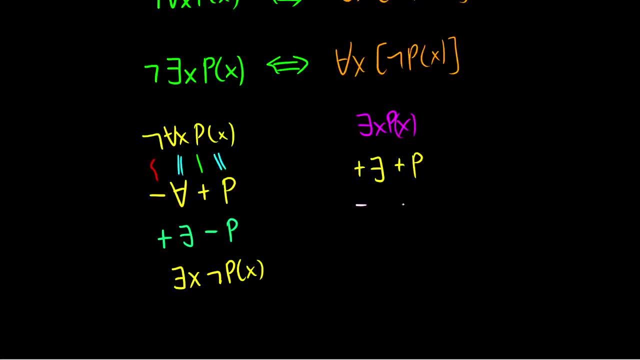 Let's flip the pluses to minuses, Let's change the existential to a universal And put a p there, And then if we rewrite this, this will be not for all. x, Not px, Which is indeed logically equivalent if we write out the definitions. 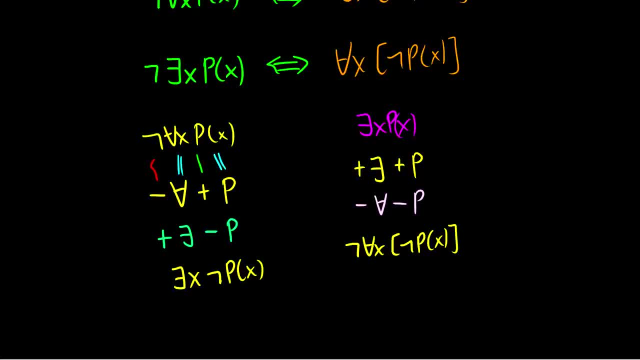 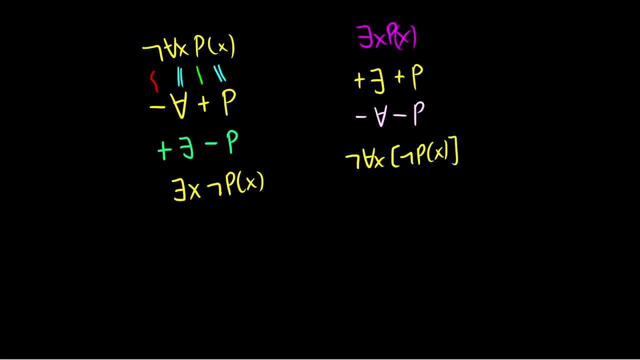 Which you can check for yourself. So that's a nice little trick you can use If you want to very quickly memorize logical equivalencies. If you ever get to modal logic in the future, You'll find that if you have something like not box p, 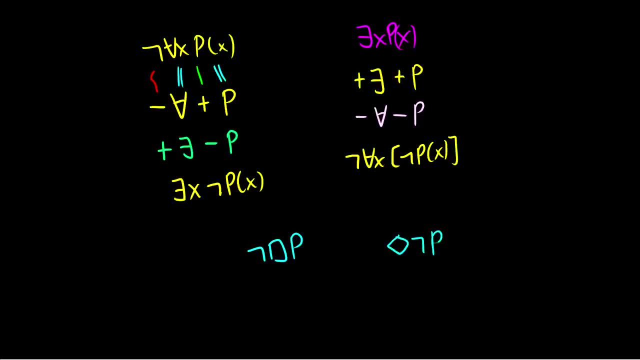 Is the same thing as diamond, not p, Which, of course, what is box and diamond? Who knows? Now, you'll find out when you get to modal logic. But this is the same thing Not. box plus p Would just go to plus diamond minus p. 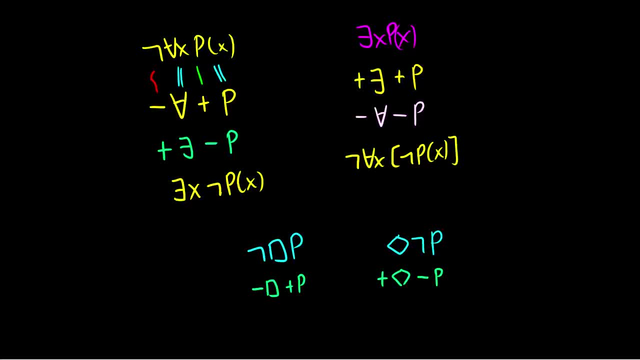 Flipping a box to a diamond And flipping the positives to negatives. These are also connected as well. So these abstract connections, Which are something that you find later in your logic career, I'm kind of throwing you at it right now So you can kind of see in advance what's coming. 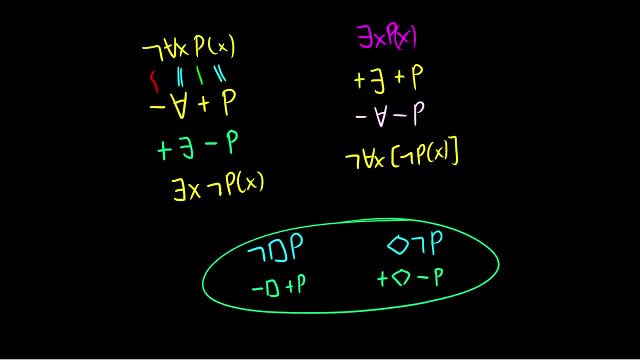 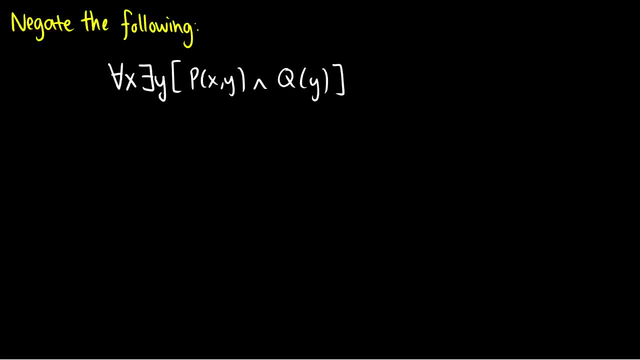 And hopefully this will help you as well in the future. Finally, Let's negate something a little bit more complicated Using the rules that we just discussed. So you might want to pause the video. Work some of this stuff out. Verify that all those equivalencies are the same. 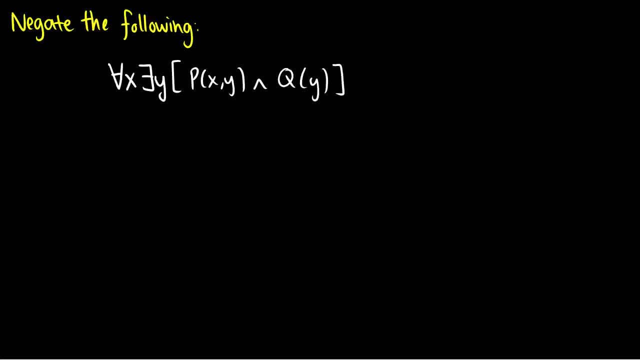 And then take a look at this, So let's negate this entire thing. Okay, so we negate quantifier by quantifier, So we can kind of think of these as having more brackets, So we can think of the brackets like this. So the first thing we want to do, 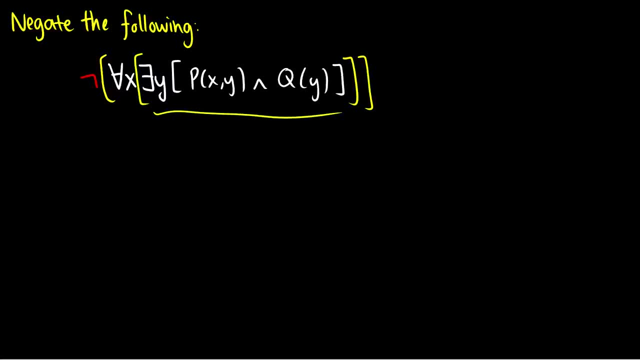 Is negate, not all x. And then there's this nonsense right there. So not all x, Blah Is the same thing as there exists an x, Not. And then the remainder of the inside, So there'd be exists a y. 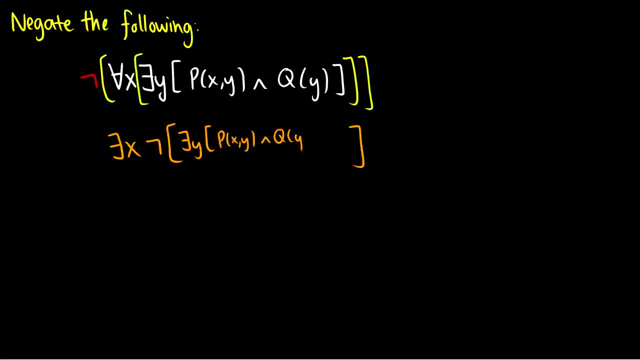 P, x, y And q, y. Okay, Now we need to negate Not exists a, y And then the rest inside, So we can leave the exists an x on the outside. Now to gate or to negate not exists y, That just becomes all y. 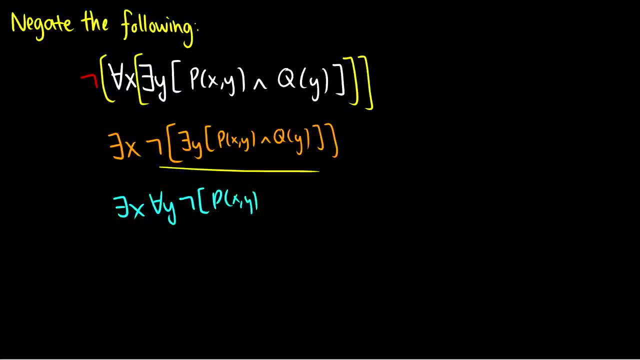 And then we get the negation Of everything on the inside. So p, x, y And q, y, And now all we do is we just do De Morgan's law And we finish it up. So exists an x, All y. 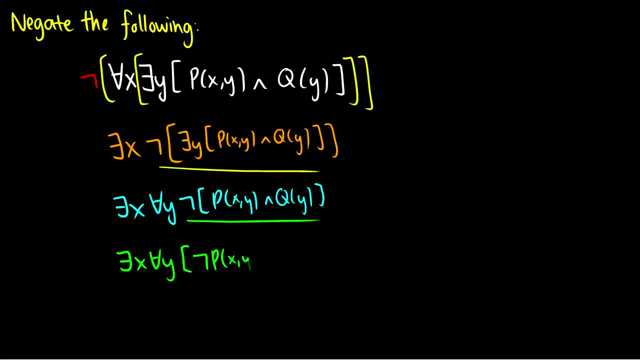 And then De Morgan's law would be not P x, y Or not q y. So that is negating. And whenever you do negation, Just take it step by step. like that: Negate one quantifier at a time. 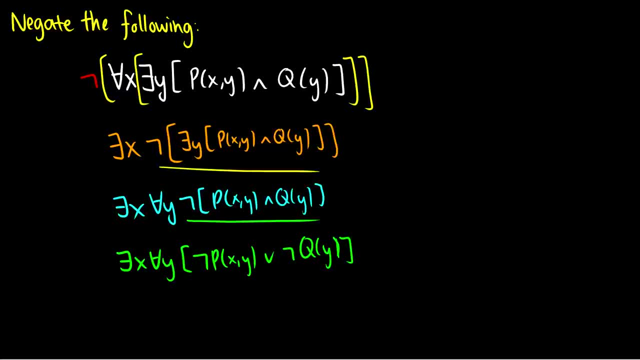 Flip the quantifier, Shove the negation through. Flip the quantifier, Shove the negation through And then do De Morgan's on the inside propositions. So that is it for logic. If you have any questions, Please feel free to ask. And I will do my best to answer them.